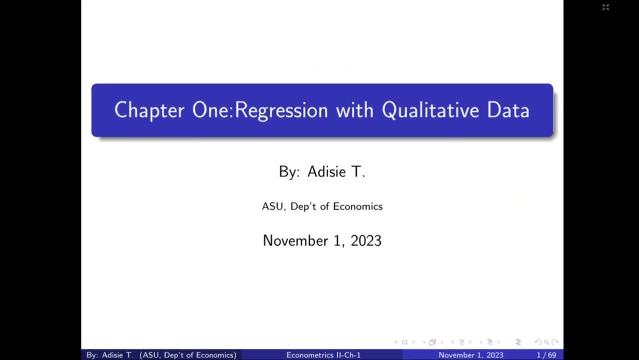 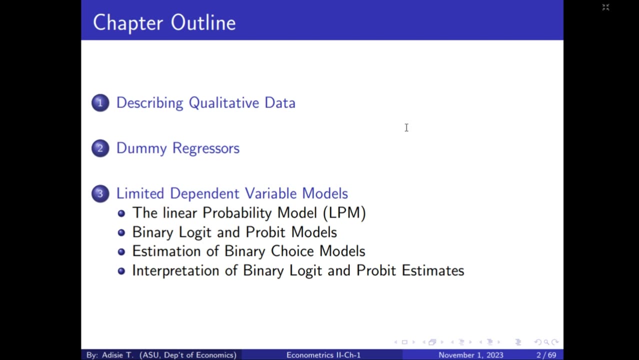 Hello, welcome to ATT Academy. In this video we will see econometrics 2, chapter 1, Regression with qualitative variables or data or regression-based dummy variables in some texts. Under this chapter we will see the nature of qualitative variables or data And then we will see how. 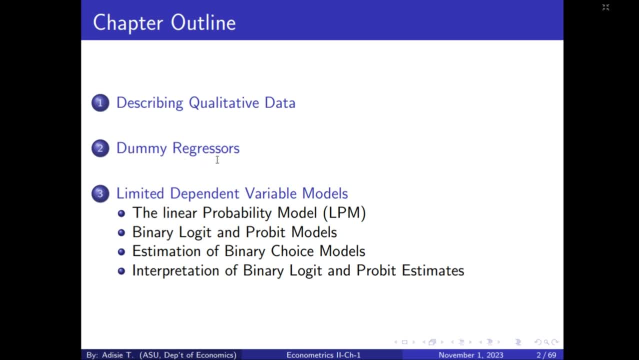 to introduce qualitative or dummy variables as independent or universal, And then we will see limit-dependent variable models. that means regression with binary choice or dummy-dependent variables. The most commonly known binary choice or limit-dependent variable models are the linear probability model, binary logit and binary probability models. First, 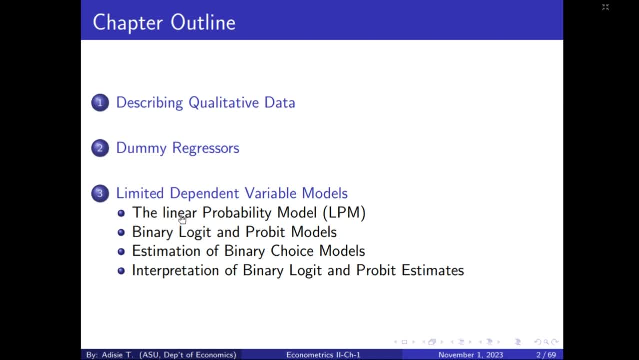 we will see the specification of these three models And the limitation of the linear probability model. The most appropriate models for binary choice or dependent variables are binary logit and binary probability models. Then we will see how to estimate binary choice model coefficients. that means the estimation method And then 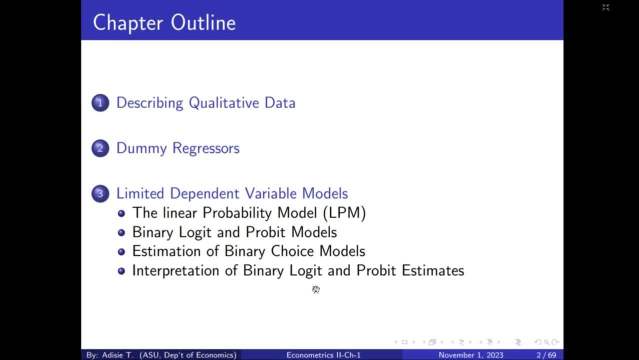 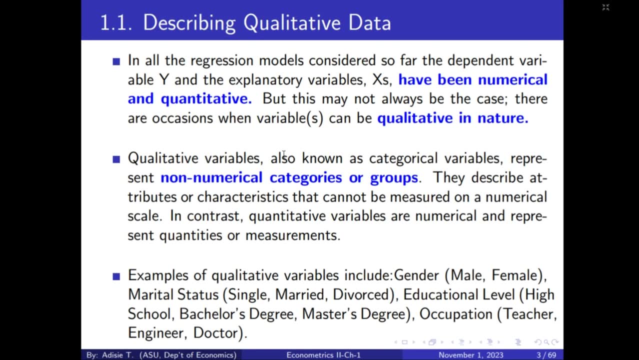 we will see how to interpret the binary choice models, specifically the binary logit and probability estimators. In all the regression models considered so far, the dependent variable y and the explanatory variables x have been nimical and quantitative. The econometrics 1 lies in the model of both. 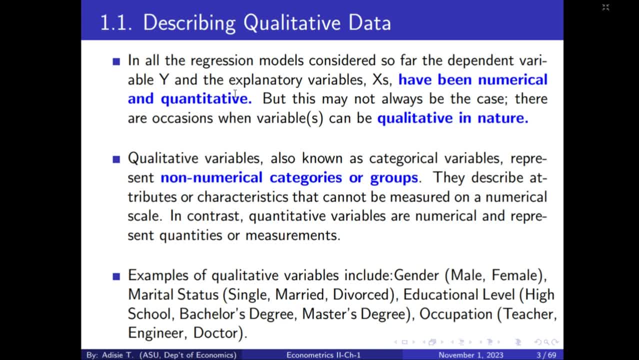 the dependent variable as well as the independent variable. Nature of quantitative and nimical number are actually not accurate, But this may not always be the case In all the regression models. what we are seeing is that quantitative andisme and quantitative also have been nimical In general. quantitative variables are the most common variable and 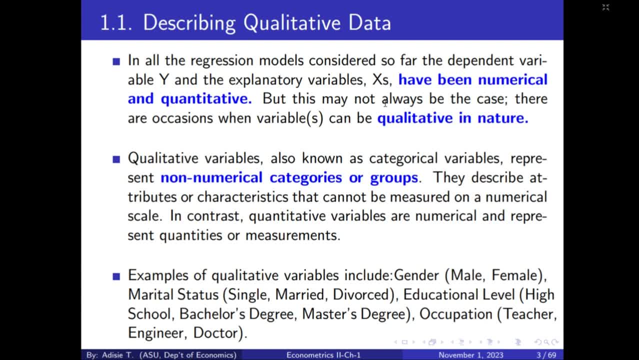 qualitative variables are not. In economics, quantitative variables live in the numerical number. That means the quantitative variables are non-economic variables. In the mathematical Income quantitative module, the group preference is not a quantitative variable, it's a qualitative variable. Qualitative variables, also known as categorical variables, represent many different categories or groups. 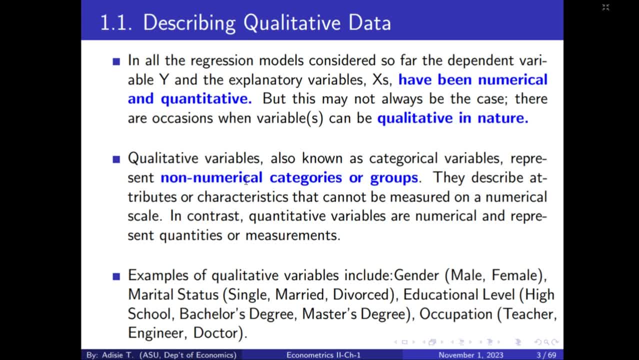 Quantitative variable means. quantitative variable means. Quantitative variable means the counting or measuring process of a group. Quantitative variable means the number of rounds: 6 rounds and 5 rounds plus 5 standard dimits or meters. Quantitative variable means the number of kilos, so the measurement process. 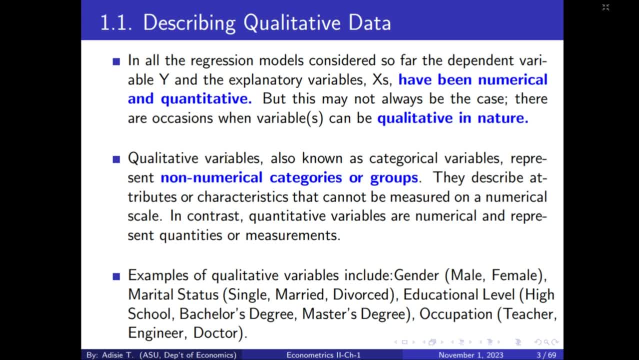 The standard dimits, or data in terms of the ratio of 8,6,7,7,8 and 12,6,8,8, and 12,6,7,8.. This is the standard dimit or data in terms of the counting procedure. 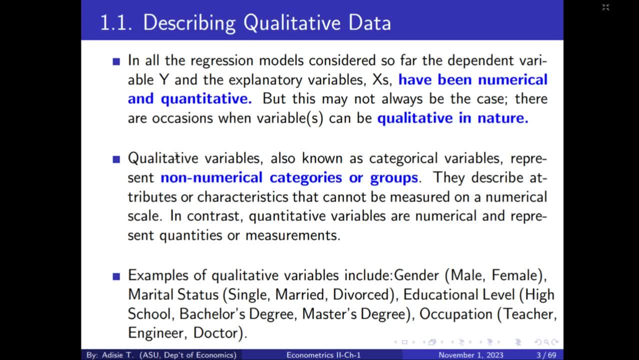 How do we do this? variables and quantitative variables. Quantitative variables is a counting procedure. in my method. it indicates another group quantity variables, for example gender variables, male, female. it is a quantity variable because it indicates the maleness or femaleness of an individual. 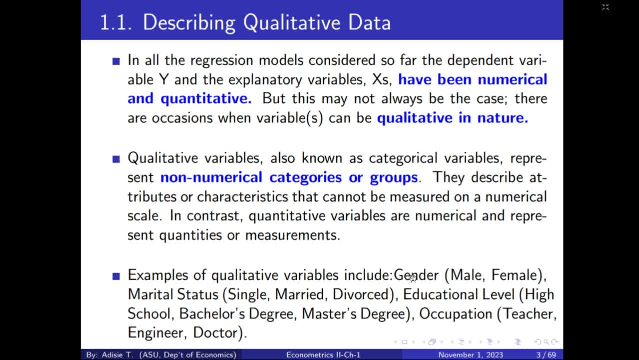 and it indicates the gender or maleness of an individual. it indicates the color of an individual. it indicates the gender or maleness of an individual. it indicates the color of an individual, attributes or characteristics that can't be measured on a numerical scale. the cardinal indicates the color of an individual. 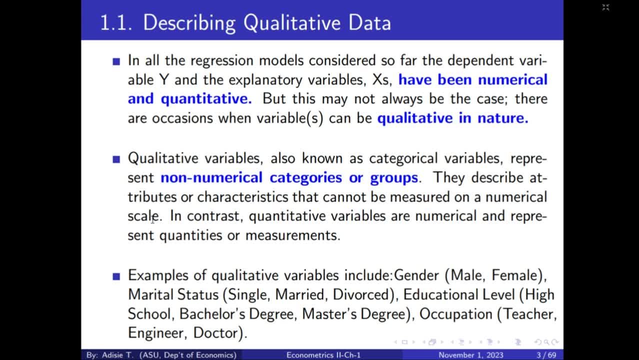 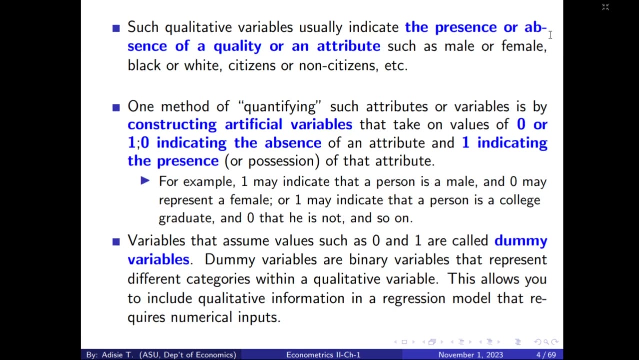 the cardinal indicates the color of the individual and the color of an individual. it is a color, a quality variable. such quality variables usually indicate the presence or absence of a quality attribute, such as, in my method, mainness or finiteness, blackness or whiteness, citizens or men. citizens- 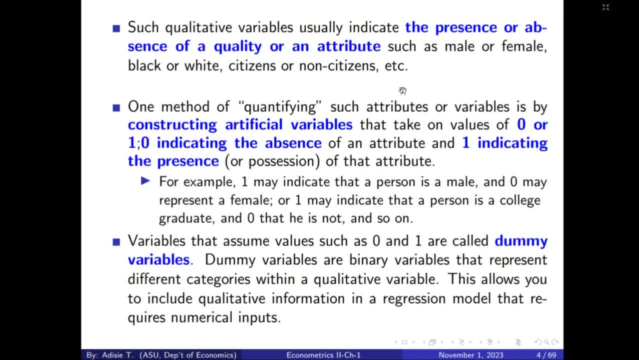 quality variables: tree, large scale, prediogram, takeaway, takeaway, double cross, cross, cross Into into learning natural, natural that are nah. So if you want to get a better picture, you can get a better picture of the quality of the variables. One method of quantifying such attributes or variables is by constructing artificial values or variables that take on values of 0 or 1.. 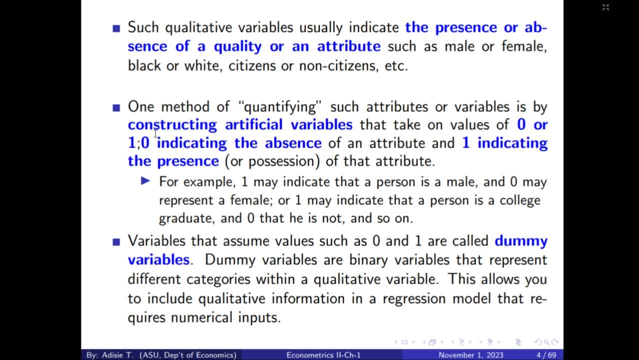 Now in statistical analysis, we can quantify the values of the variables And always represent them. For example, if an event appears or presents, 0 will be the record. If an event appears, 0 will be the absence, So 0 will be the absence. 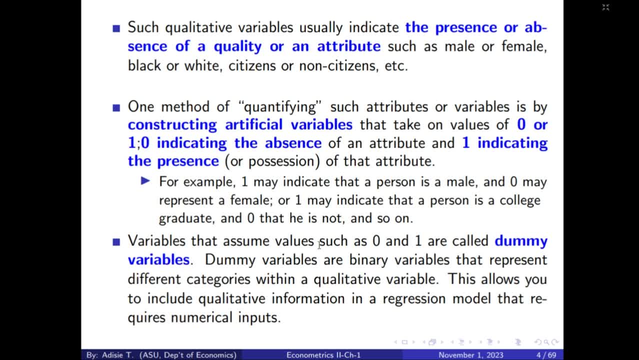 And it will be the present. It is a matter of success. Values ie 0 and 1 are called tamii variables. So another value, 0, represents the tamii variables. Tamii variables are binary variables. Binary variables are the previous variables. 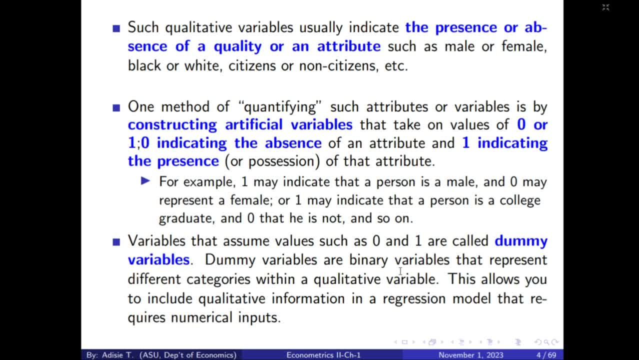 So our answers are the absence and the present success-failure blurb. So the variable in the model is Binary. It represents different categories within a qualitative variable. This allows you to include qualitative information in your evaluation model that requires numerical inputs. 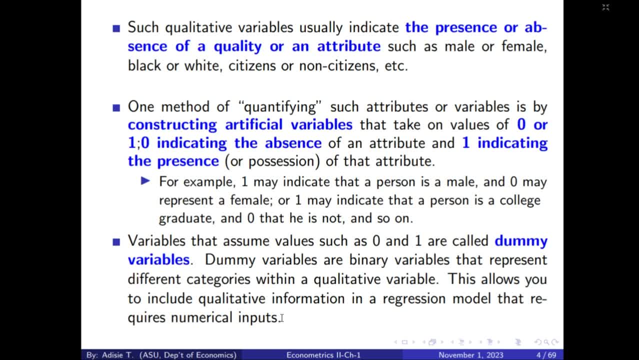 The quality variable is called the Demi-variable. It represents zero. The quality variable is called the independent variable. So the quality variable is called the Demi-variable. The regression analysis is called the independent variable, Demi-regressors or Demi-variables. 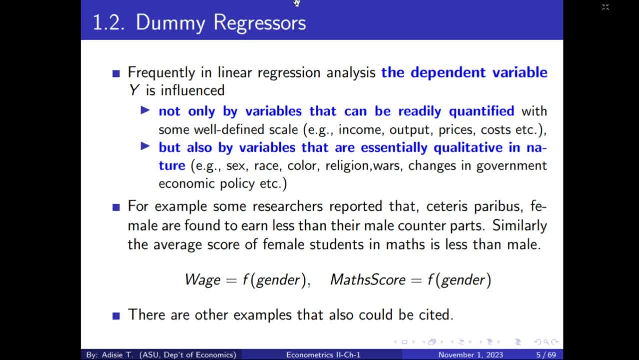 Demi-variables as independent variables. Frequently, in linear regression analysis, the dependent variable Y is influenced not only by variables that can be readily quantified on a semi-defined scale, but also by variables that are essentially qualitative in nature. These four variables are qualitative in nature. 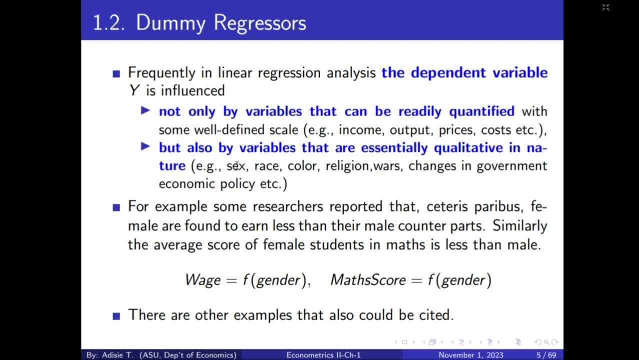 They indicate the presence or absence of an attribute: Sex, maleness, femaleness, Race, some race, Color, some colors, Religion, the religions that we know. Wars with the war, without war, Change in government policy before the change in government policy and the end after the change in government policy. 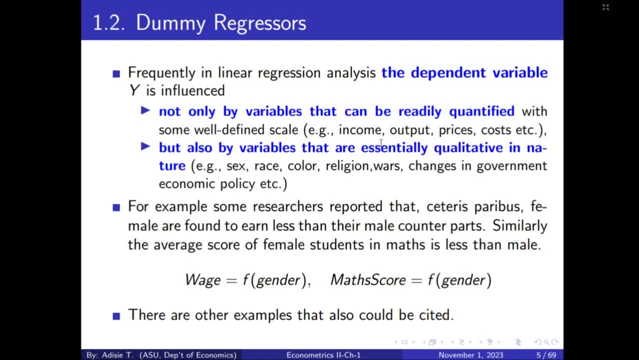 So these four variables are qualitative in nature, But these ones are quantitative. They do have their own structure. They do have their own standard. US income: It can be measured in the dollar Outputs. The amount of output produced It can be quantified in kilograms. 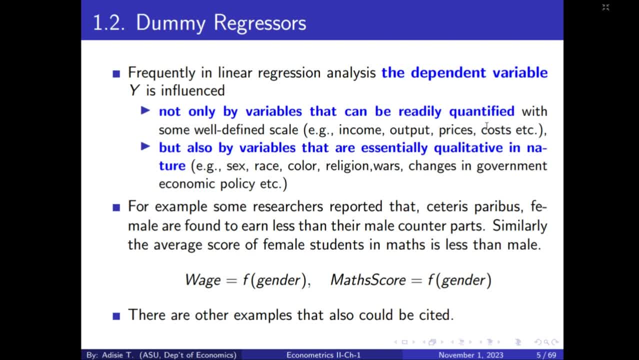 Or the amount of the units Price. It is a quantitative But these are qualitative. So many variables, even variables, determine numeric possibility And like, for example, some researchers reported that stress variables- females are found to earn less than their male counterparts. 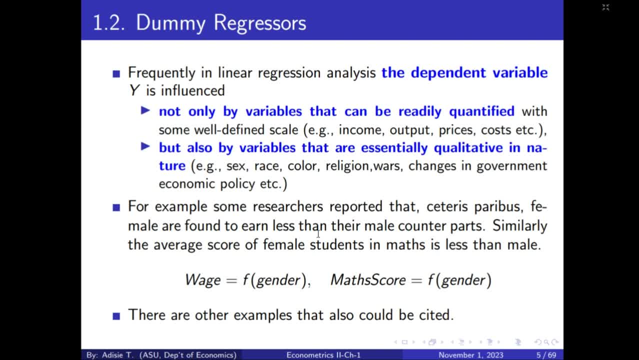 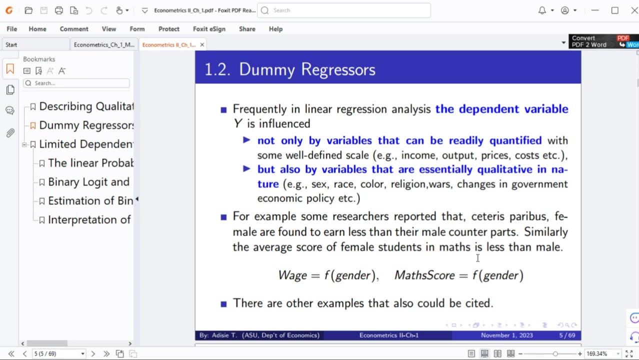 So these are quantitative. Andि ário ユーファンタジー. Yaw 증 P, north curve. Yaw C lorsque gestures are over. so that's why we have to use math score to find the answer. 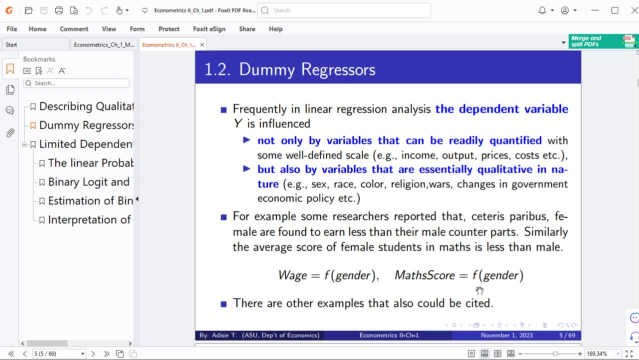 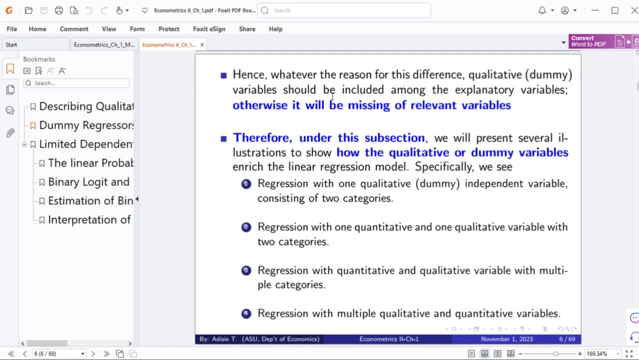 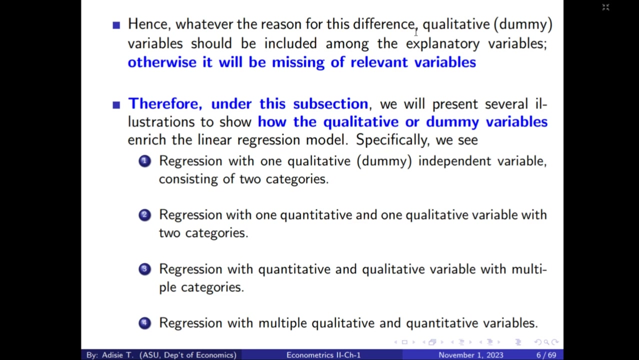 so that's why we have to use math score to find the answer. so math score is math score bars according to general number. another example that could be size. we can use the quantitive variable to find the answer. so what is the reason for this difference? you can see the scale is divided into series. 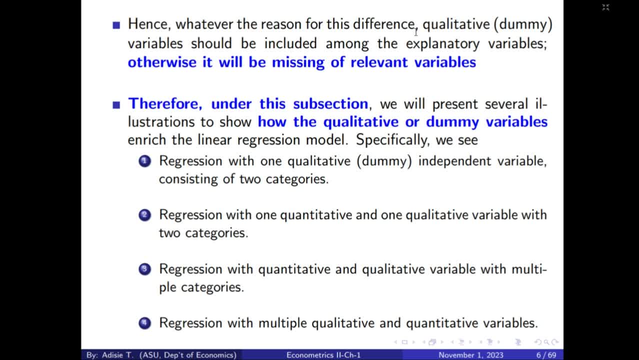 if you use the same variable, there will be a difference. if you use the similar variable, then the difference will be visible. if you use the same variable, then the difference will be visible. So, in the end, pain variables are introduced regardless of the quality, whatever the reason for this difference. 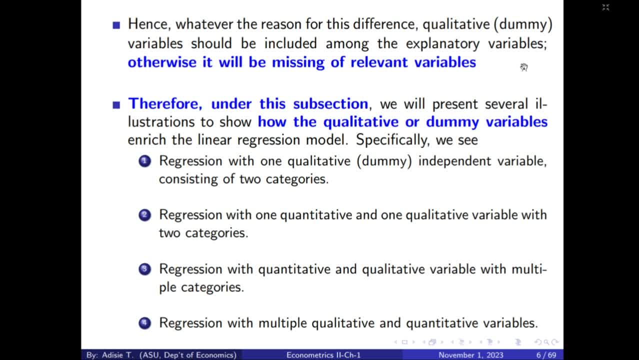 the quality of the pain variables should be included among the explanatory variables, Otherwise it would be missing of relevant variables. In my case the relevant variables are missing in the model. So missing of relevant variables is a consequence of Econometrics 1, Chapter 4,. 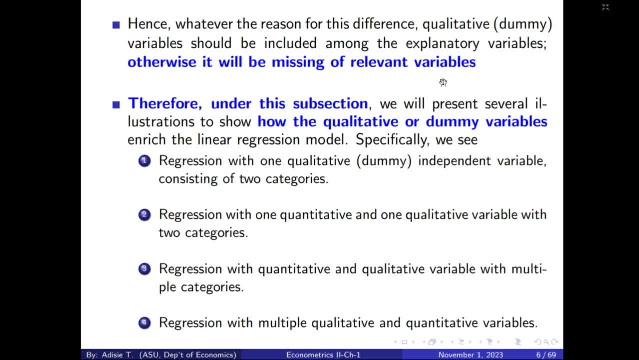 like in the model, ALS should be as dense and consistent in the model. So in my case, the quality variables and the independent variables are missing. Therefore, under this subsection we will present several illustrations to show how the quality of pain variables enrich the linear regression model. 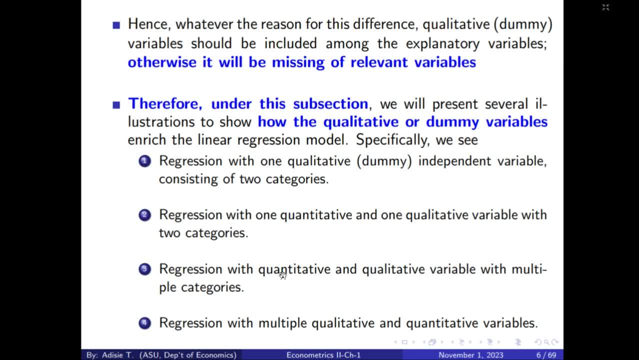 Specifically, we see step by step that we can understand the model and that the model can be applied in the model. Regression will be one. The quality of the pain variable consists of two categories. That means the quantity of the pain variable as a function of 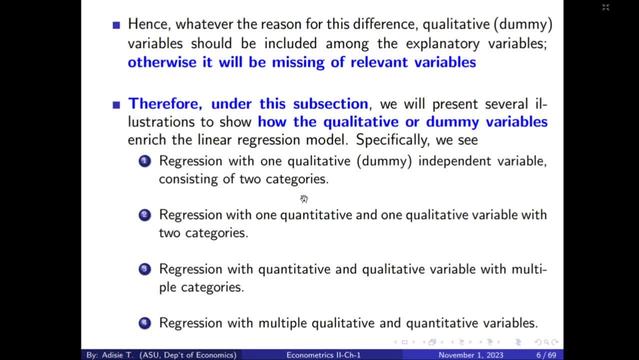 and the quality of the pain variable, with two categories: The weight as a function of the math score, as a function of the gender, the sex and the language. Now the regression will be one quantitative variable and one qualitative variable, with two categories. 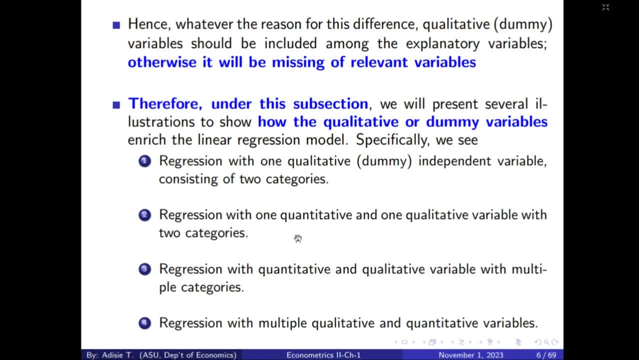 It is very much determinable. The one quantitative variable contains two variables And the function of the two variables is: the first variable is quantitative, The second variable is the qualitative. The second variable is the qualitative variable And how the quality of the pain is determined.